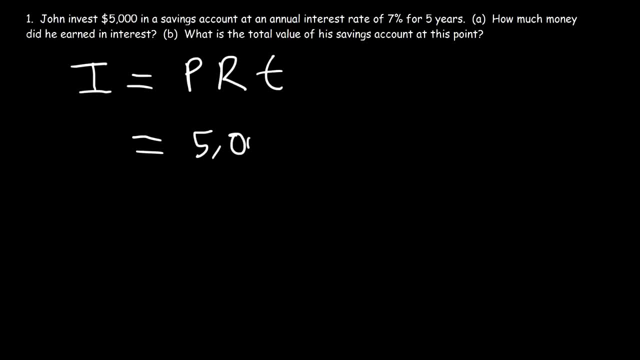 P is the principal, that's how much money he invests in the account, which was $5,000.. R is the annual interest rate, which is 7%, but in the form of a decimal. The decimal form of 7% is 7 divided by 7.. 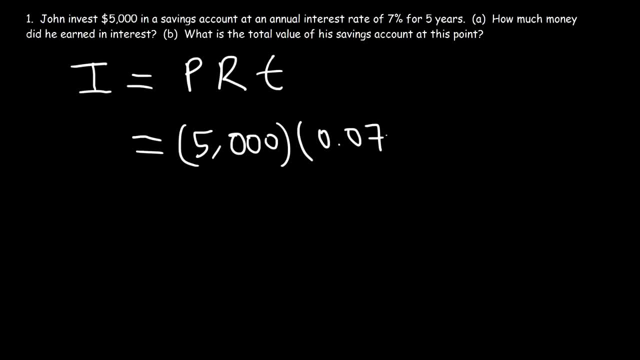 7 divided by 100, which turns out to be .07.. And T is the time in years, So T is 5 years. So all we've got to do is take 5,000, multiply it by .07, times 5.. 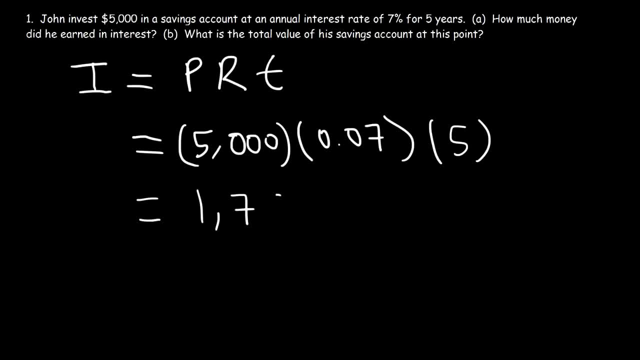 So he receives a total of $1,750 in simple interest. Now part B: What is the total value of his savings account at this point? So keep in mind he initially put in $5,000, and his account was credited with $1,750 in interest. 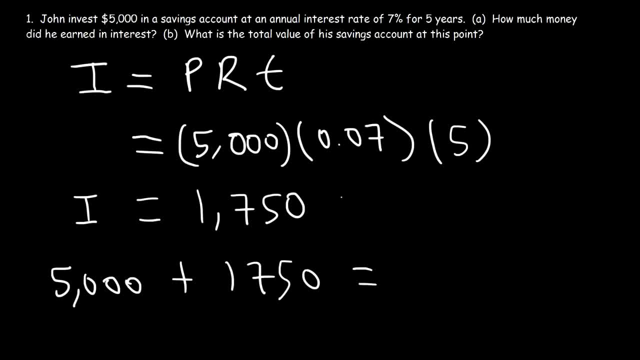 So his total account value at this point is $6,750.. So that's how much money he has in the account at the end of 5 years using the simple interest formula. So this is the answer for part B And this is the answer for part C. 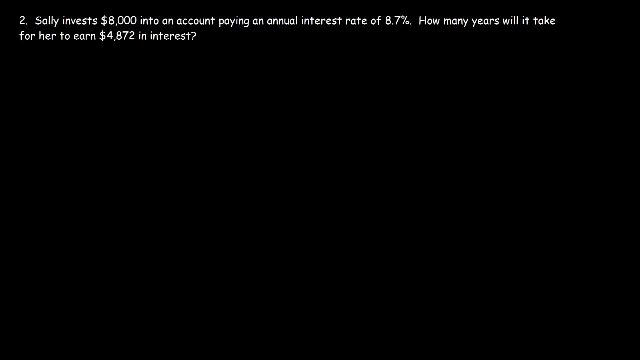 And this is the answer for part A. Number two: Sally invests $8,000 into an account paying an annual interest rate of 8.7%. How many years will it take for her to earn $4,872 in interest? The equation that we need to use once again is: I is equal to PRT. 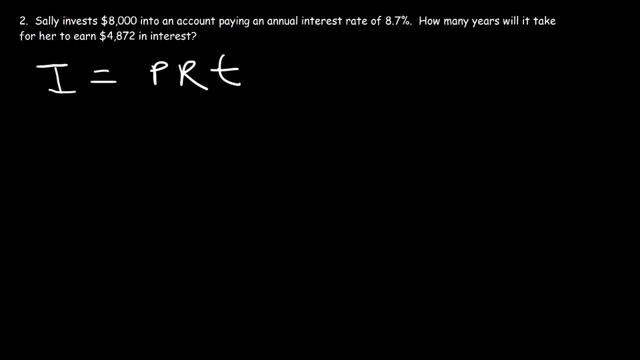 So the interest that she earned In these years are $4,872.. The principal, the amount that she puts in the account, is $8,000.. That's P. R is the interest rate. So if we take 8.7 and divide it by 100, R is .087.. 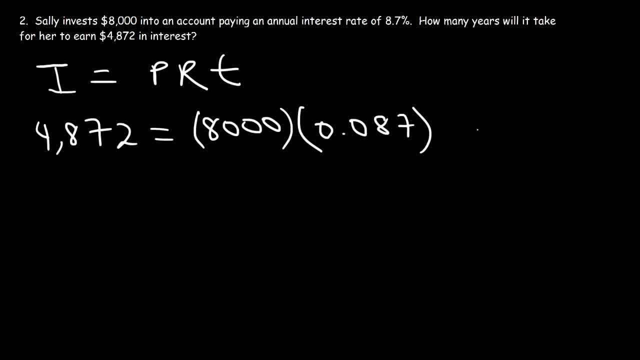 That's the decimal equivalent of 8.7%. Our goal is to find T. We need to find the value of T in this problem Because we're looking for How many years it's going to take her to earn this level of interest. 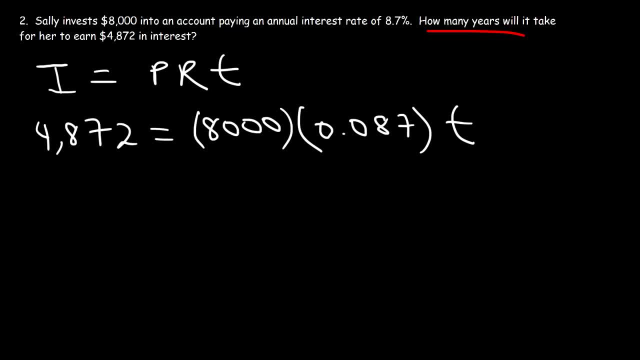 So the first thing we need to do is multiply 8,000 by .087.. Which is 696.. Now the next thing we need to do is divide both sides by 696.. So 4,872 divided by 696.. That's 7.. 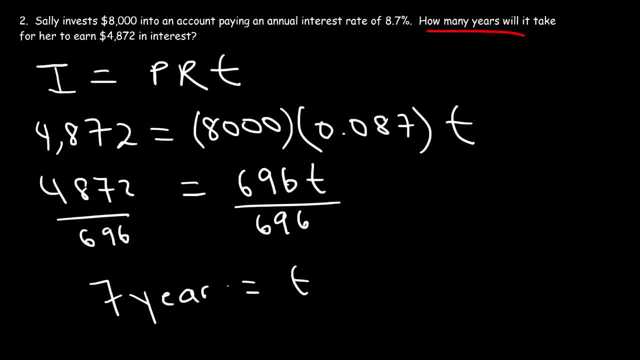 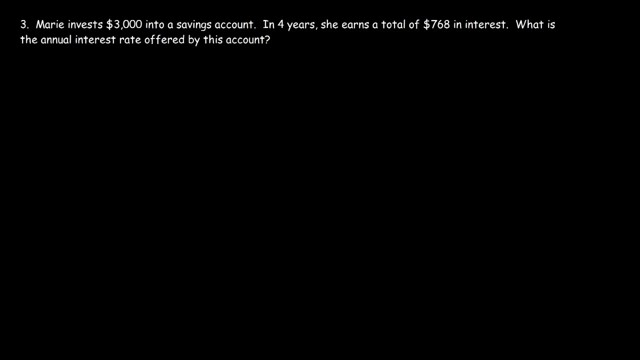 So therefore, it's going to take her 7 years to earn $4,872 in interest If she invests $8,000 into an account paying an annual interest rate of 8.7%. Number 3,, Mary invests $3,000 into a savings account. 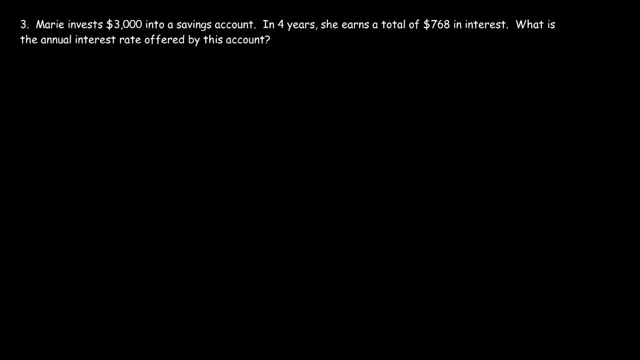 In 4 years she earns a total of $768 in interest. What is the annual interest rate offered by this account? So we're going to use the same formula Now in this problem: what's I, what's P, what's R and what's T? 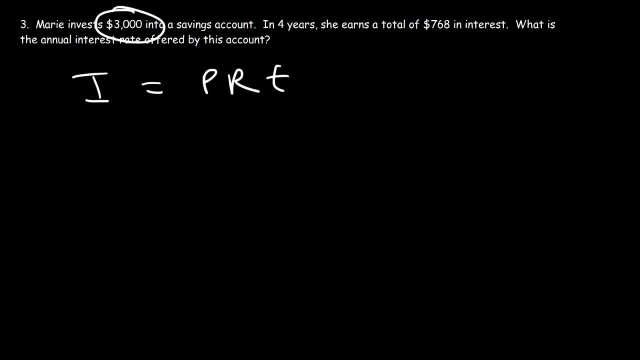 The 3,000 is the amount of money she puts into the savings account, So that is the principal. The $768 is the interest, So we can replace I with that number. Now we're looking for the annual interest rate, So we need to find the value of R. 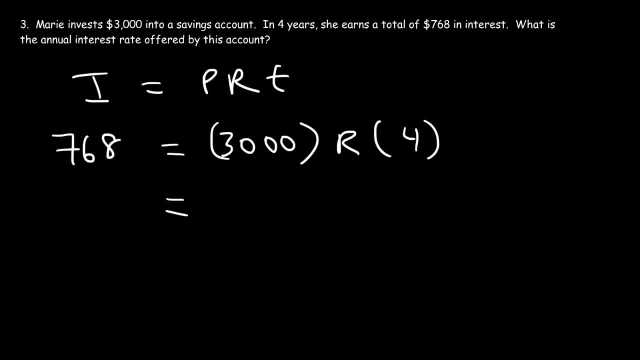 T is 4.. So first let's multiply 3,000 by 4. That's going to be about 12,000.. Now the next thing that we need to do is divide both sides by 12,000 to isolate R. 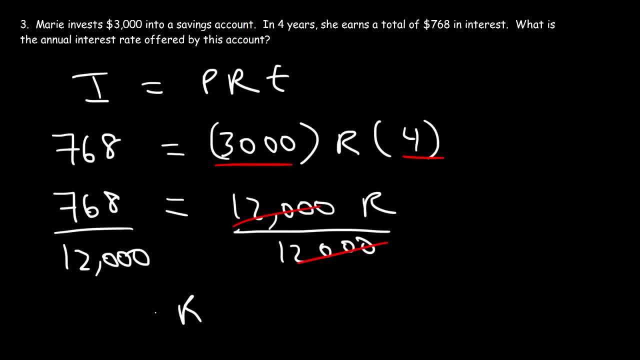 So R is going to be 12,000.. I mean it's going to be 768 divided by 12,000.. So as a decimal that's 0.064.. To convert this into a percentage, multiply by 100.. 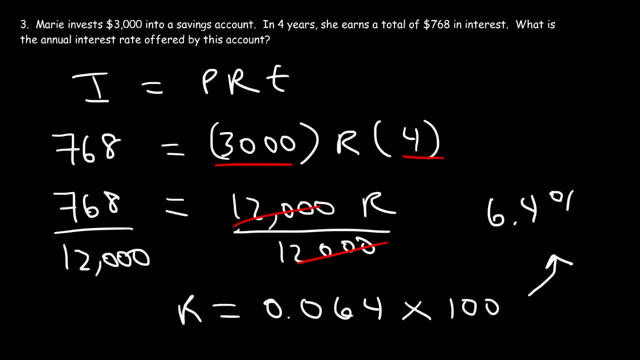 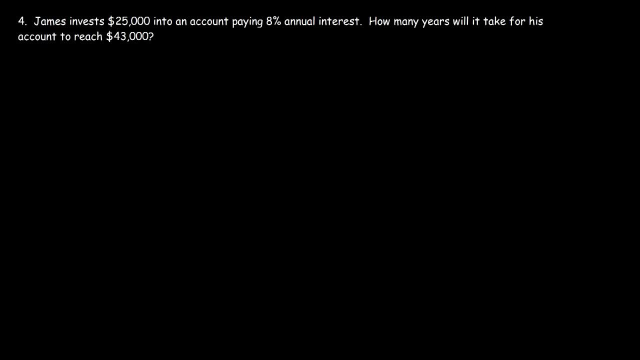 So the interest rate is about 6.4%. So that is the annual interest rate offered by this account. Number four. James invests $25,000 into an account paying 8%. How many years will it take for his account to reach $43,000?? 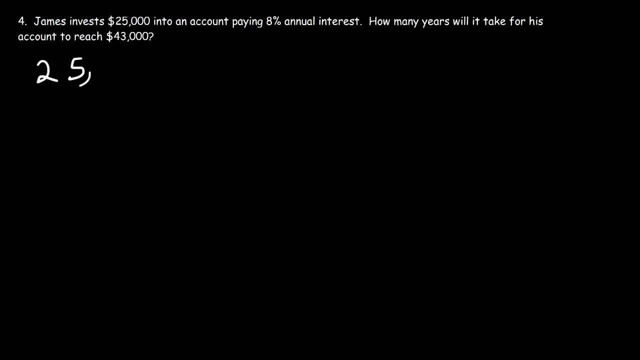 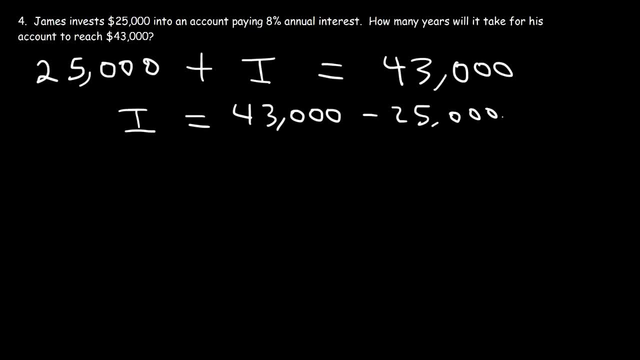 And $43,000 is the difference between $43,000 and $43,000.. So if we subtract those two numbers you should get $18,000.. So that's how much money he's receiving in interest in this time period. 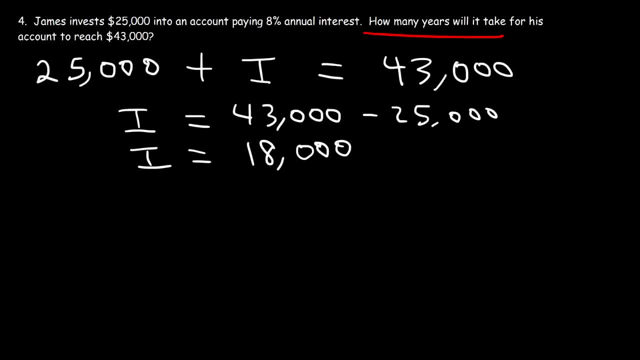 And we've got to find out what that time period is. So our goal is to find T. How many years will it take for his account to reach that level? So, using this formula, I is equal to PRT. We have the interest earned, which is $18,000. 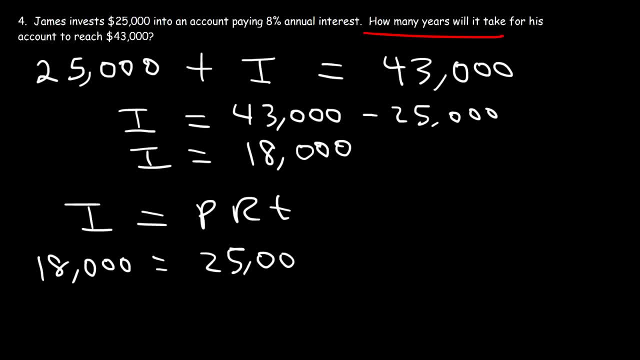 Starting with a principal of $25,000.. The annual interest rate is 8%. 8 divided by 100 is .08.. So our goal is to find the value of T. So first let's multiply 25,000 by .08.. 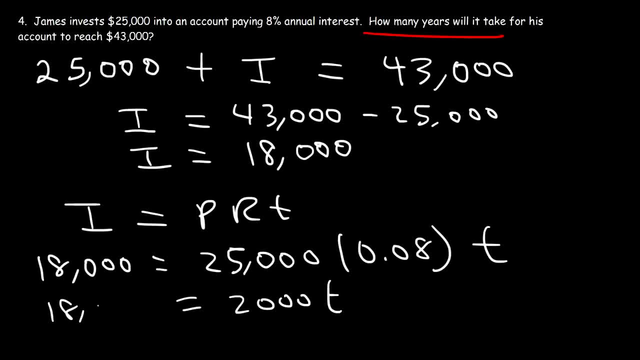 So you should get 2,000.. And now let's divide both sides by 2,000.. So 18,000 divided by 2,000.. We can cancel the three zeros, So it's equivalent to 18 divided by 2, which is 9.. 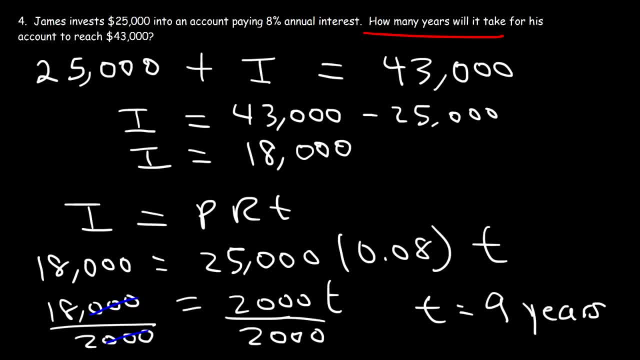 So it's going to take 9 years for his account to go from $25,000 to $43,000.. If he's receiving an 8% annual interest rate, So it takes 9 years to earn $18,000 in total interest. 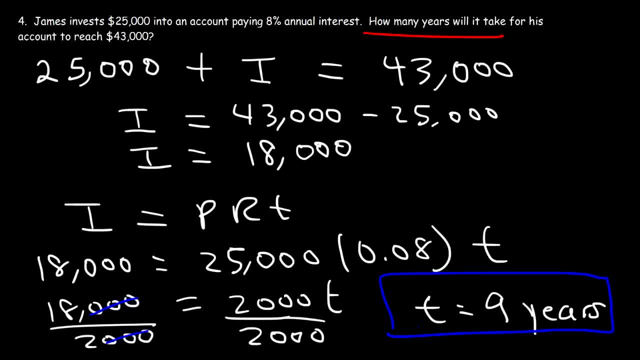 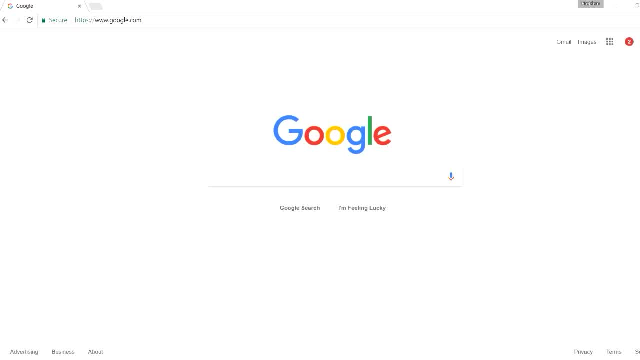 So that's it for this video. So now you know how to use the simple interest formula to solve problems like this. Now I want to show you one of my algebra courses that might be useful to you if you ever need it. So go to udemycom. 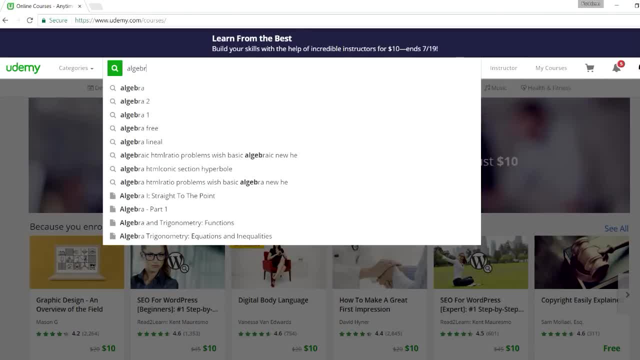 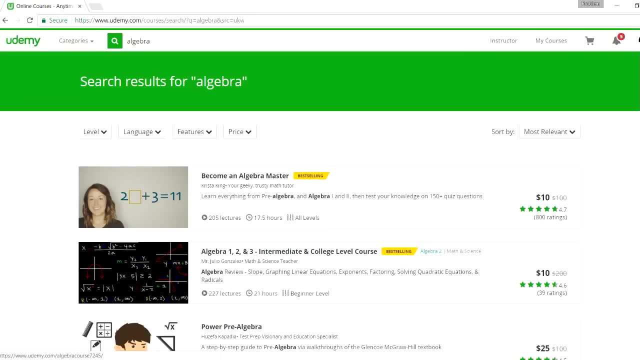 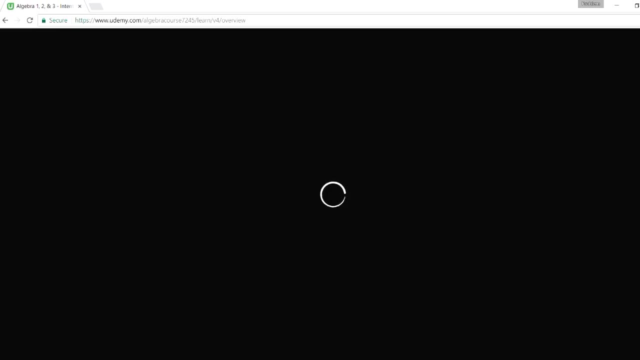 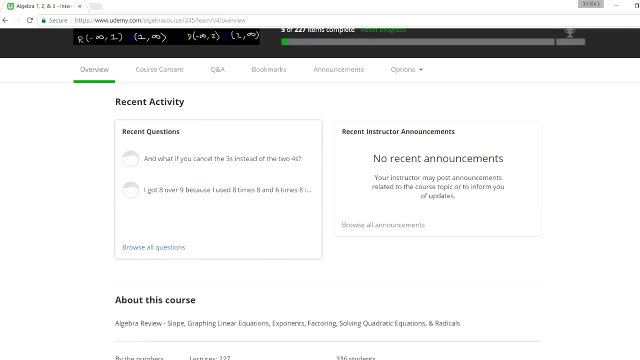 Now in the search box, just type in algebra and it should come up. So it's the one with the image with the black background, Okay, Okay. So if you select that option and if you decide to go to course content, you can see what's. 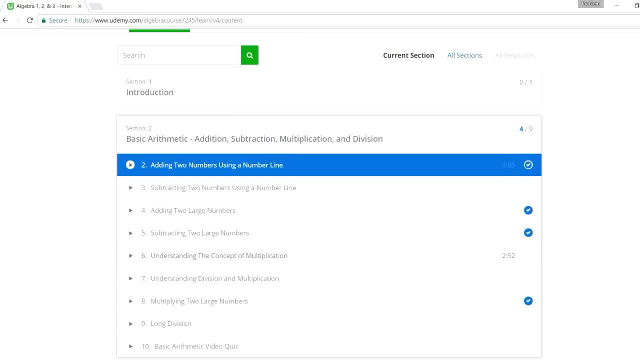 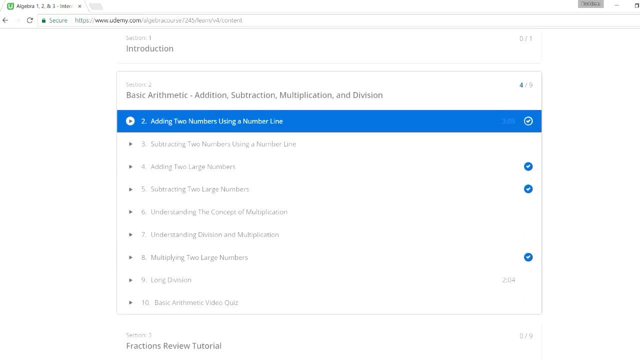 in this particular course. So the first section, basic arithmetic- for those of you who want to focus on addition, subtraction, multiplication and division, And it has a video quiz at the end. It's a multiple choice video quiz. You can pause it, work on the problems and see the solution. 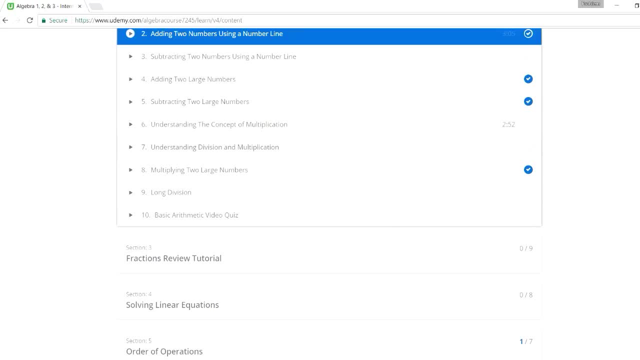 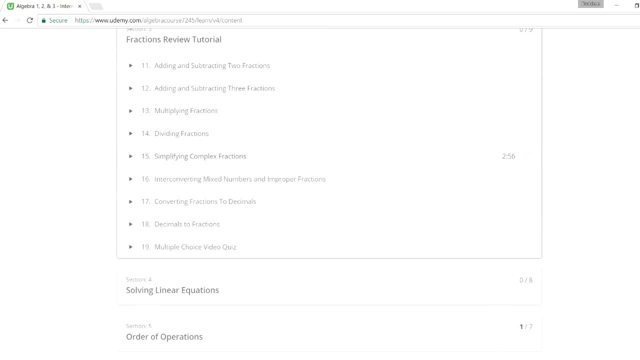 It covers long division, multiplying two large numbers and things like that. The next tutorial is on fractions: Adding and subtracting fractions, multiplying and dividing fractions, converting fractions into decimals and so forth, So you can also take a look at that. 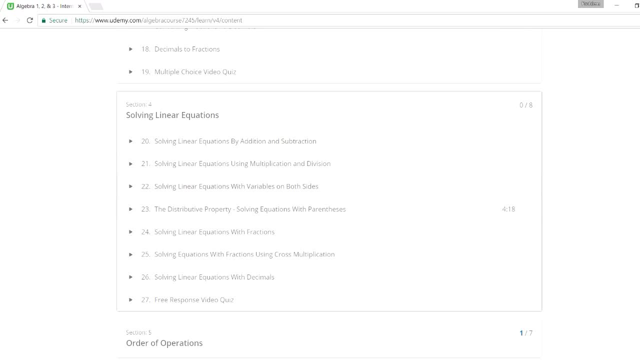 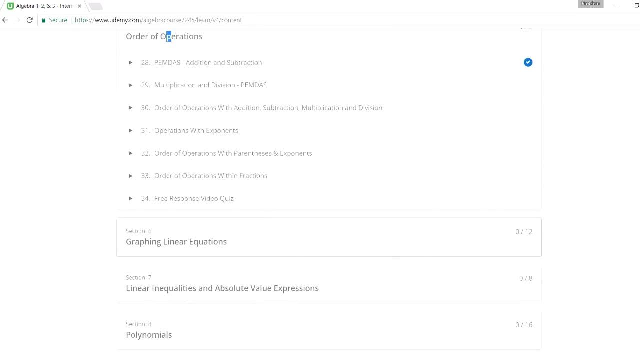 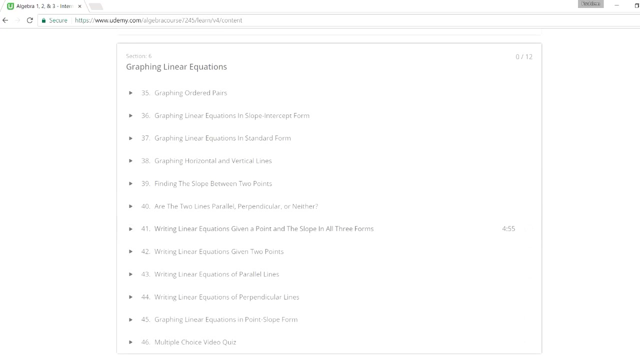 Next, solve the linear equations which we covered, And just more examples if you need more help with that. The next topic, order of operations, which is also useful: Graph and linear equations. Okay, You need to know how to calculate the slope. you need to be familiar with the slope intercept. 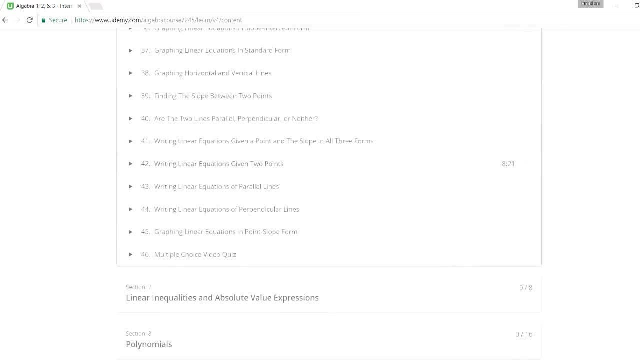 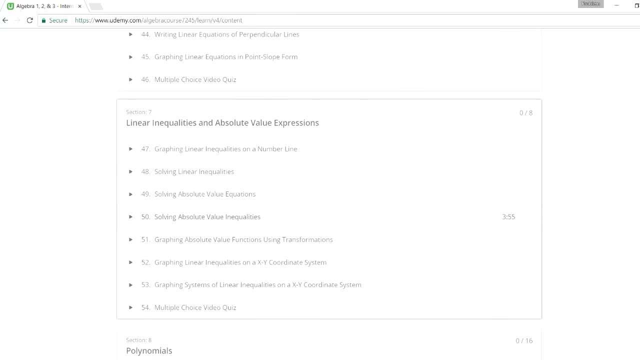 form, standard form and just how to tell if lines are parallel, perpendicular and so forth, And there's a quiz that goes with that as well. The next topic is on inequalities and absolute value expressions, which are also seen in a typical algebra course. 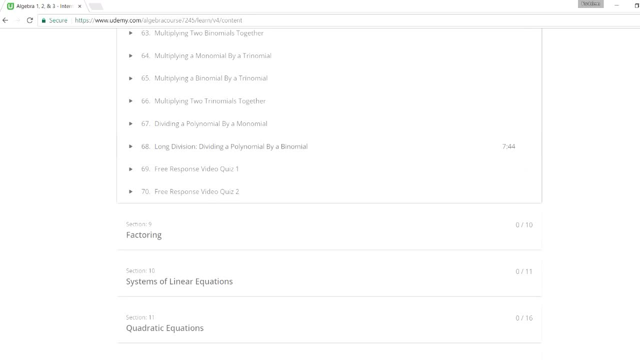 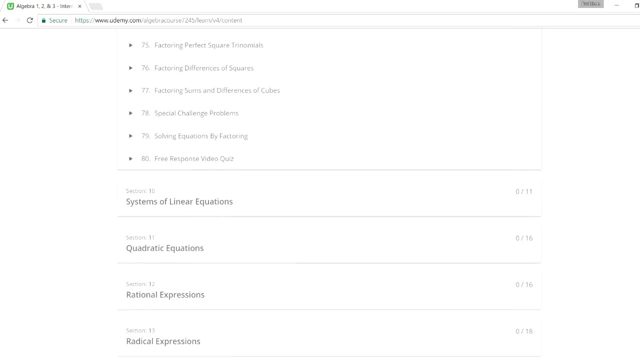 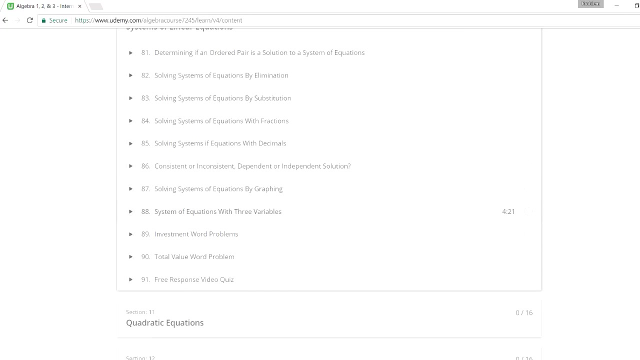 And then we have polynomials, and that's a long section, And then factoring- That's another topic you need to master- And then system of equations. You can solve it by elimination, substitution. there's also word problems as well. 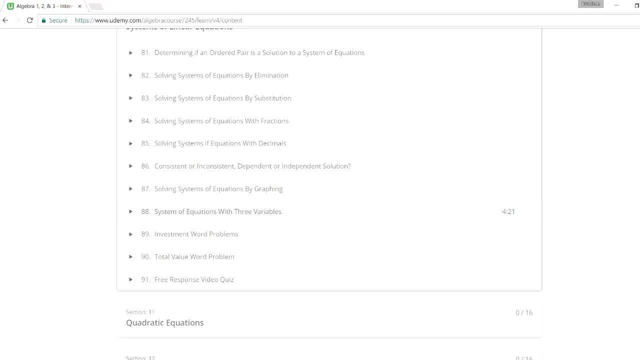 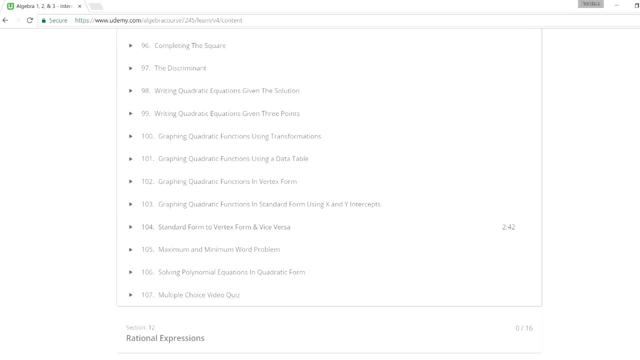 Sometimes you've got to solve equations with three variables- x, y and z- so that could be helpful. Next, quadratic equations: how to use a quadratic formula, how to graph them, how to convert between standard and vertex form, And then you have rational expressions.